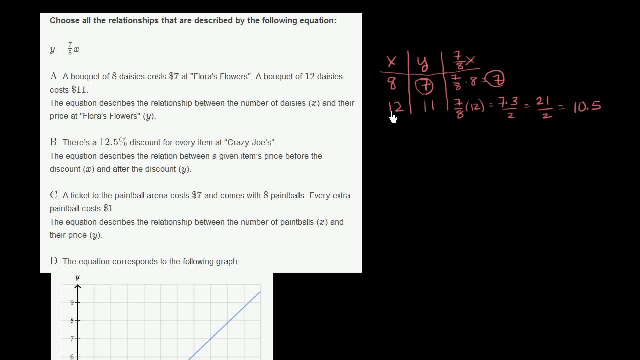 So if y were equal to 7 eighths x, 12 daisies would cost $10.50.. But we just learned that 12 daisies cost $11.. So these two things aren't equal to each other, Aren't equal to each other. 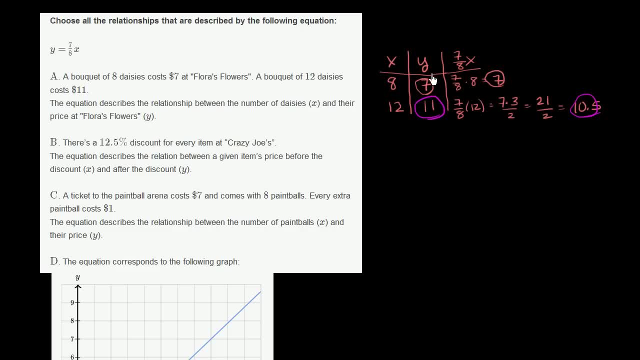 So this is not the same relationship. In this scenario, y does not equal 7 eighths x, So we can rule this one out. Let's look at relationship B. There's a 12.5% discount for every item at Crazy Joe's. 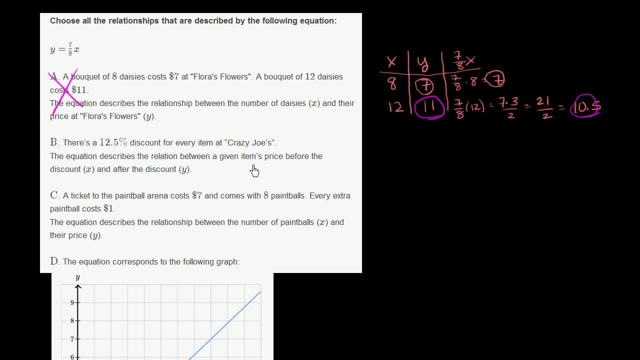 The equation describes the relationship between a given item's price before the discount and after the discount. So here they're giving us a percentage And this equation- right over here it's written as a fraction, So let me at least convert this into a fraction. 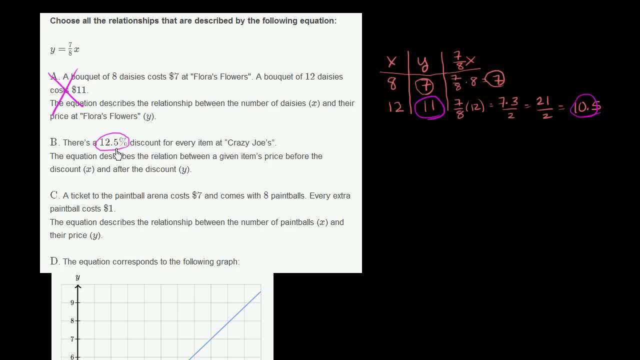 and see what kind of a fractional discount this is, And maybe I can construct an equation and see if that equation is the same as this one here. So 12.5% is literally the same thing. So 12.5% is the same thing as 12.5 over 100.. 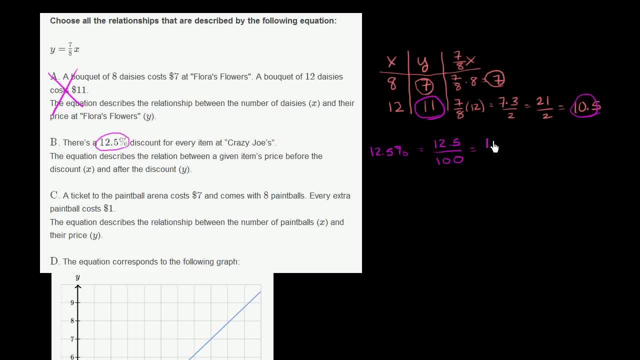 And if we multiply the numerator and denominator by 10, that's the same thing as 125.5.. Let's see if we can simplify this a little bit. If we divide the numerator by 125, we get 1.. We divide the denominator by 125, we get 8.. 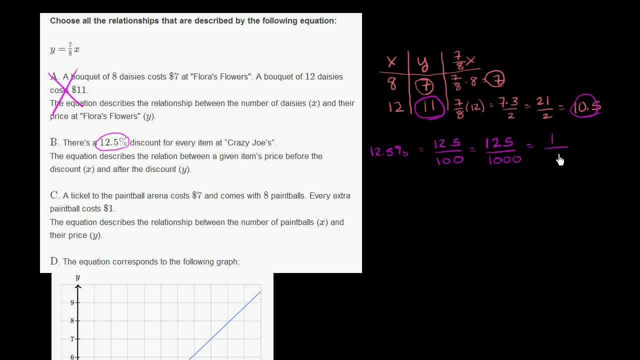 8 times 125 is 800 plus 200, which is 1,000.. So this is the same thing as 1 eighth. So there's really a 1 eighth discount for every item at Crazy Joe's. The equation describes a relationship. 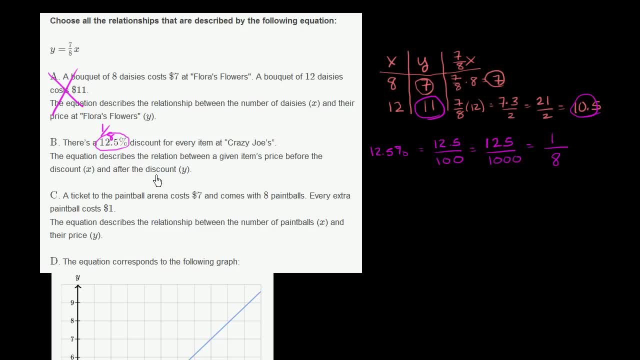 between a given item's price before the discount and the price after the discount. So let's just think about that: The price after the discount, based on the information they gave here, is going to be equal to the price before the discount minus the discount. 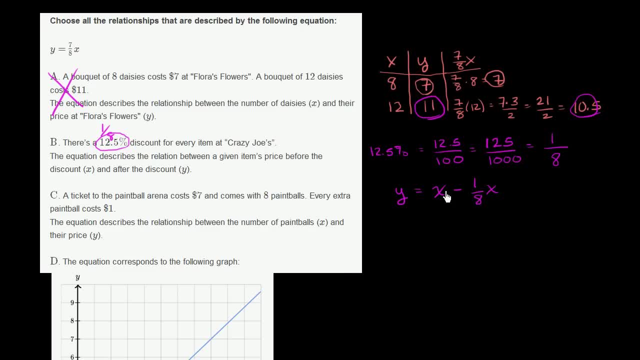 so minus 1 eighth of the original price. Well, what's x minus 1 eighth x? Or another way of thinking about it, what's 1x minus 1 eighth x? Well, that's just going to be 7 eighths. 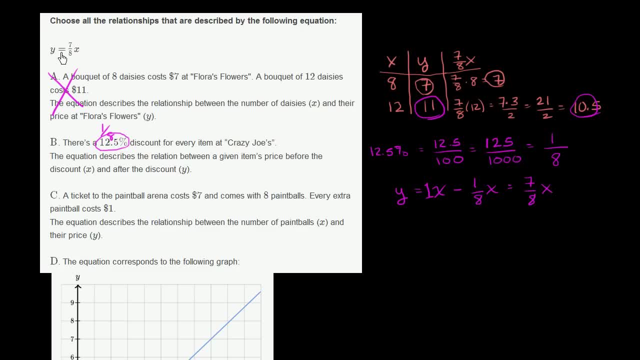 So this relationship is the exact same as this one over here. The price after the discount is 7 eighths of the original price, So we can feel good about this one. These two are the same. Let's look at scenario c. 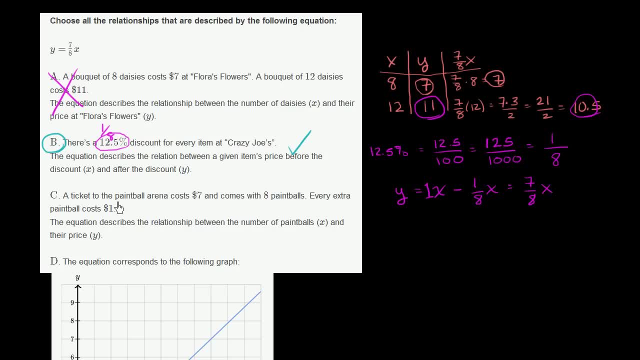 And I will do scenario c in orange. A ticket to the paintball arena costs $7 and comes with 8 paintballs. Every extra paintball costs $1.. The equation describes the relationship between the number of paintballs x and their price. 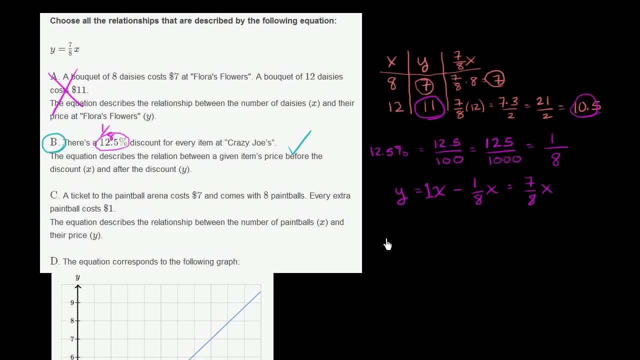 their price, y. So let's look at this. We'll do something similar to what we did up here, So we'll have x, which is the number of paintballs, And then we have y, which is their price, And then we will think about what 7 eighths x. 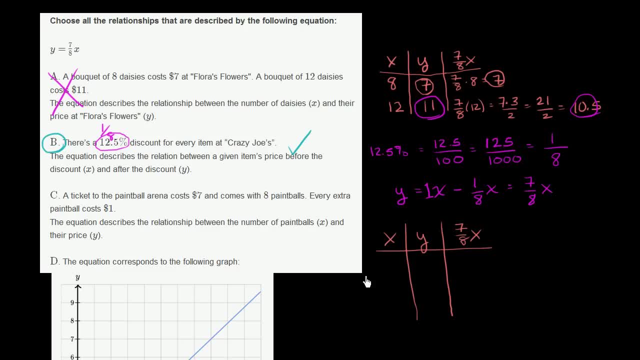 would have been equal to: And let's see if y is equal to 7 eighths x. So when we get 8 paintballs, so x is the number of paintballs. So when we get 8 paintballs, the price is 7.. 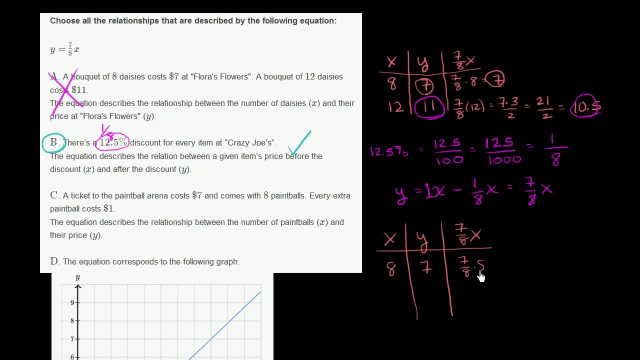 And if we take 7 eighths x, so 7 eighths times 8 is indeed 7.. So in this scenario, for this data point, it is true that y is equal to 7 eighths x. Now let's get a couple of other data points. 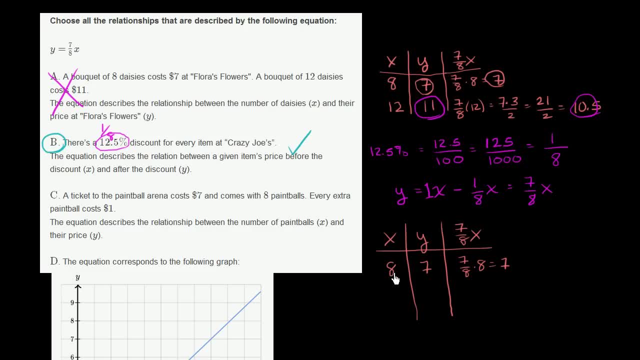 And we might have to construct these. So every extra paintball costs $1.. So if we have one extra paintball- so we have 9 paintballs- we're going to have to pay $1 more. We're going to have to pay $8.. 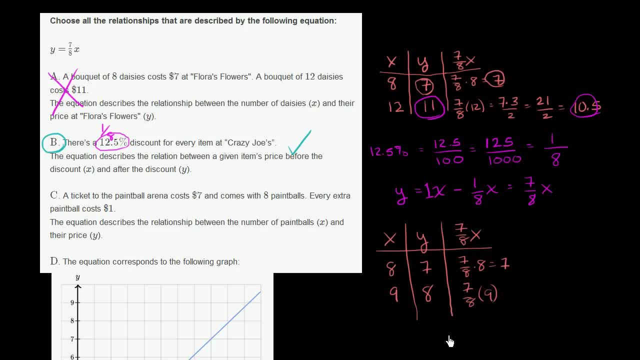 And so what's 7 eighths x here? So 7 eighths times 9.. Well, we don't even have to compute it. This is going to be something that's going to be like 63 over 8.. 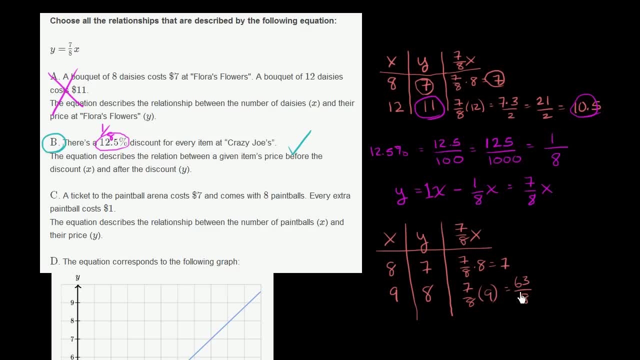 64 over 8 would be 8.. So this is a little bit less Then, a little bit less than 8.. But the important point is that 8 is not equal to 63 over 8.. y does not equal 7 eighths x in this scenario right over here. 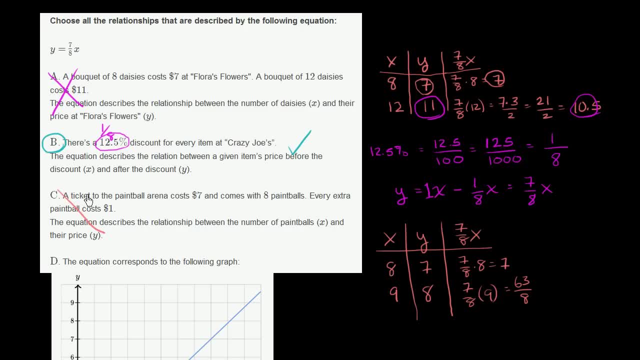 So this equation does not describe all of these data points, So we can rule that out. Finally, they say the equation corresponds to the graph following graph. So let's see if y equals 7 eighths, x corresponds to this graph right over here.